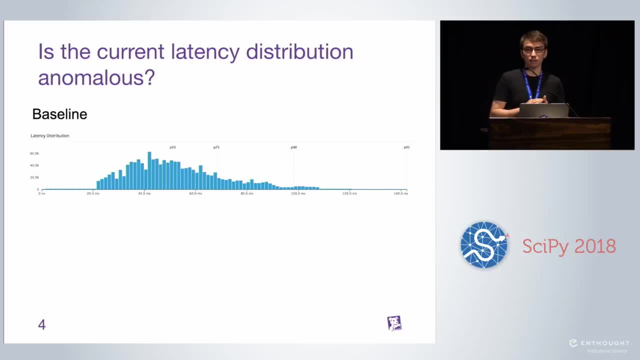 constitute this baseline from a timeframe during which we know that nothing wrong happened in the infrastructure or in the application. And then we look at the distributions of latencies over the last minute. Here's what we get, And here we can clearly see that there is a shift towards the higher values. So qualitatively we can. 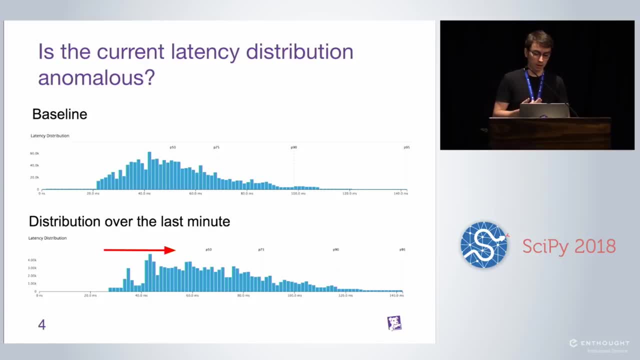 say that there is an anomaly here. But this is only a qualitative observation And we need a quantitative way, a technical way, to say that it is anomalous, And so the first idea that we might have is working with sample statistics. So, very basically, we can look. 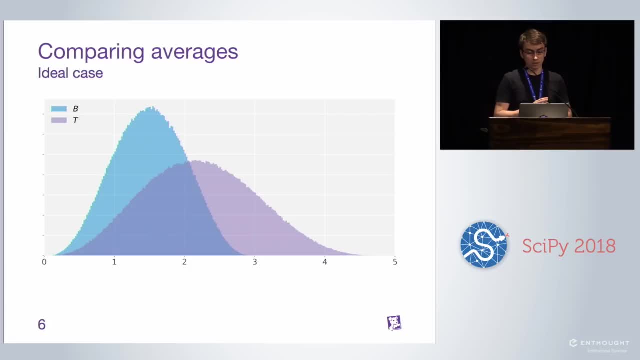 at the average of the distribution. So here we have our two distributions, B, which is the baseline, and T, which is the distribution, And if we look at the average of both of them, it's clear that the average for T is significantly lower. 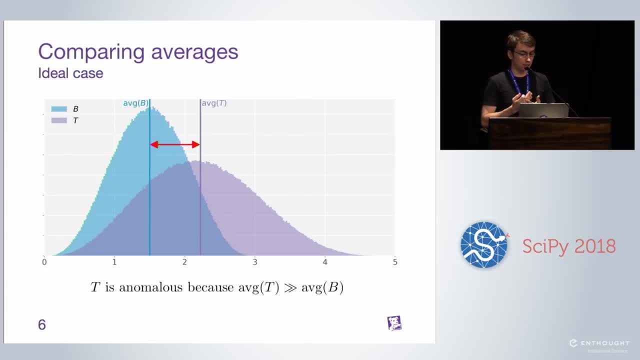 It's significantly higher than for B, So we can flag this test distribution as anomalous. We can have a threshold of 1.2, for example, And if the average of T is 1.2 times at least higher than the average of B, then we flag this as anomalous. Of course, this is not going to work in all cases. 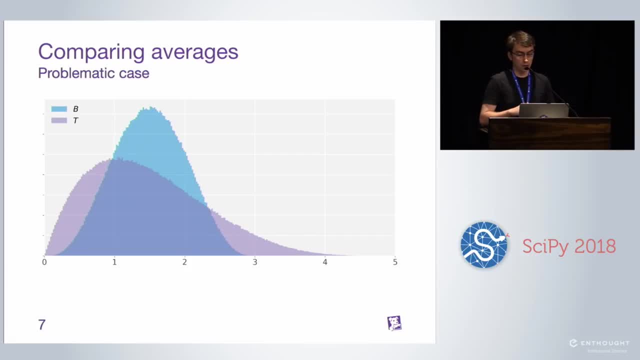 So, for example, we might have distributions that don't have the same shape, And here we can see that for the test distribution, we have a significant share of requests in the tail That takes more time than usual, So we should flag this as anomalous. However, if we 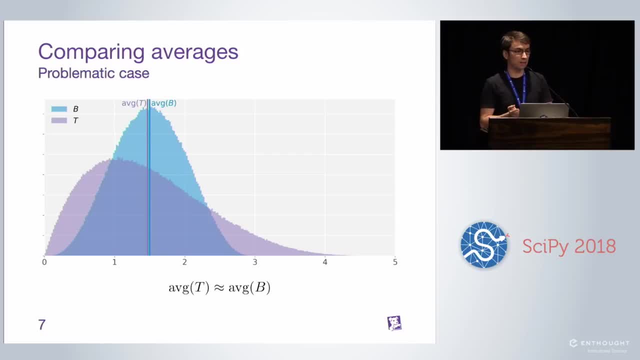 take the average, we get almost the same, So the average is not correct here. to detect this anomaly, We could imagine using the maximum of the distribution, but we will have issues when we have long tails And so when there is, for example, one single request that for some reason took much more. 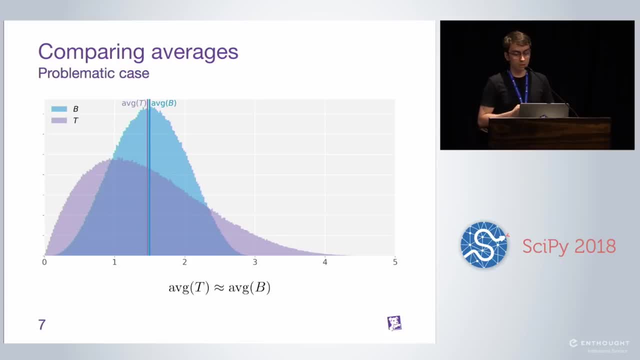 time than the rest. So the maximum might not be great, but we can still take some percentile We can. what's commonly used is the 95th percentile. So if we look at the 95th percentile of this distribution, we see, we do see the difference. 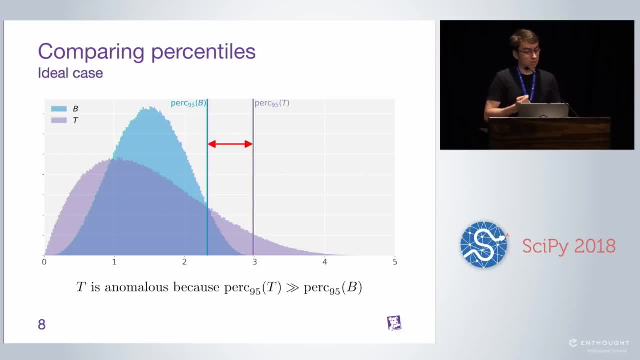 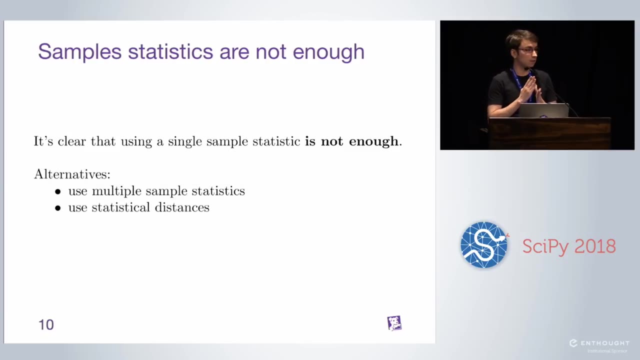 and we can flag the test distribution as anomalous. But you probably imagine what the next slide is. We can still imagine distributions that don't have the same shape, but still the percentiles are the same. So at this point it's clear that using a single sample statistic is not enough to detect exhaustively. 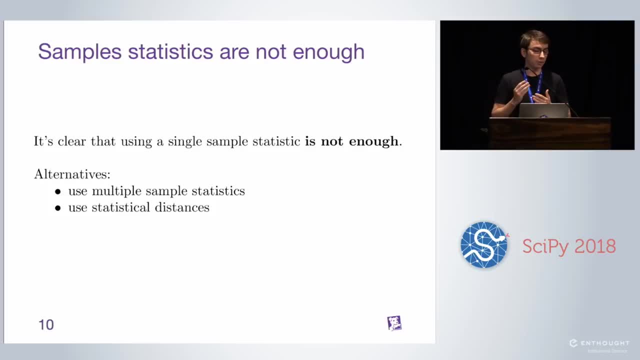 all the anomalies. So what we could do is using multiple sample statistic. Maybe we can combine the anomalies, Maybe we can average the maximum to some percentiles. but then we have to come with a criterion to merge all those sample statistic and say whether or not we should consider. 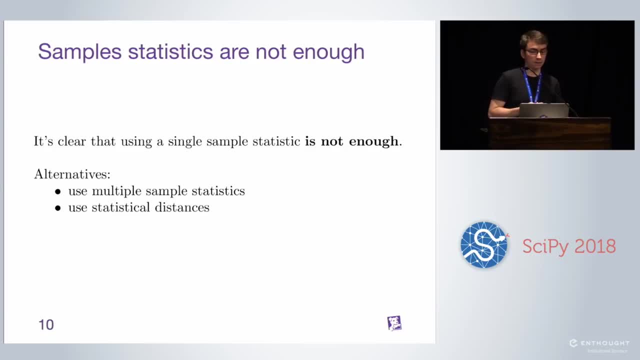 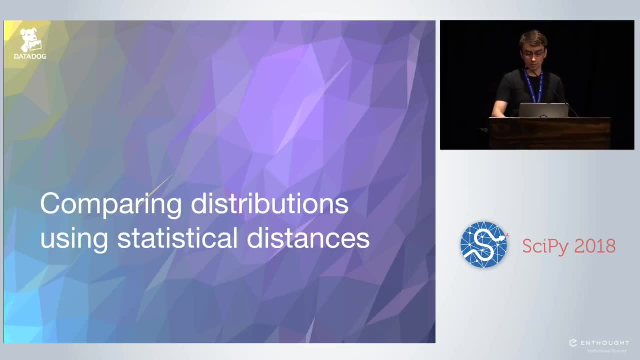 the test distribution as anomalous, Another solution is to use statistical distances. So, in short, statistical distances are distances between statistical objects, And to explain that, I start with something that's commonly known, which is the Kolmogorov-Sminov. 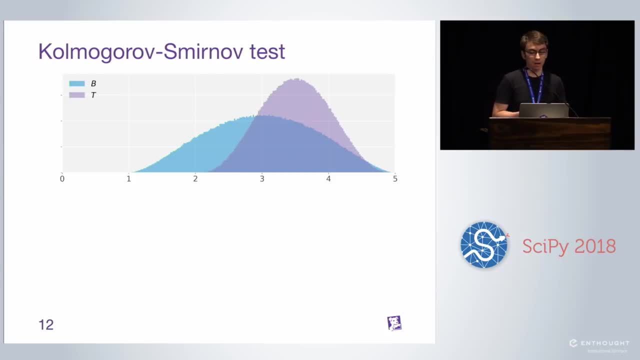 test. So this is a statistic. It's a statistical test that's commonly used to say whether a sample is drawn from a reference distribution or whether two samples are drawn from the same distribution. So we consider the latter case here. So we have our two distributions here. 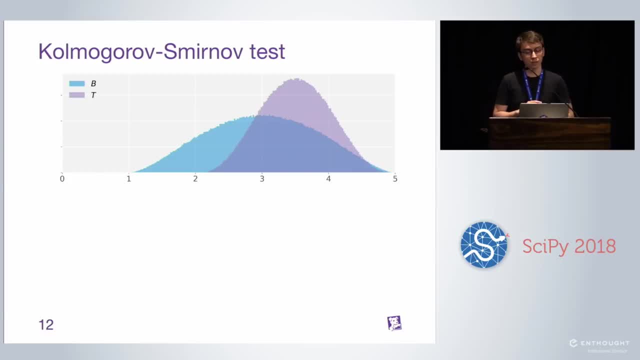 And the way how the Kolmogorov-Sminov test usually works. you would plot the cumulative distribution function. You would consider the maximum difference, absolute difference, between the cumulative distribution functions. This would give you a number. You would have a number between zero and 1.. 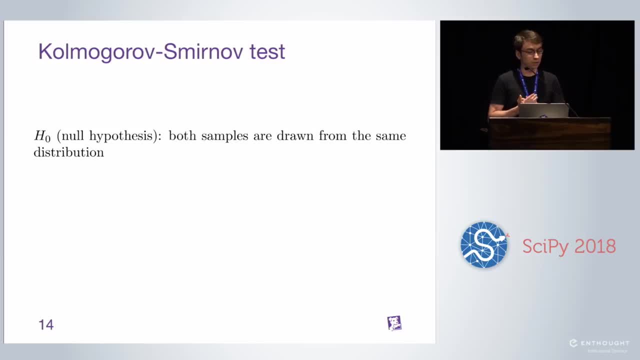 And then what you would usually do is considering the null hypothesis H0,, which is that both samples are drawn from the same distribution. You would have a critical value at significance alpha. So, based on how confident you want to be on the test, you would use that critical value. 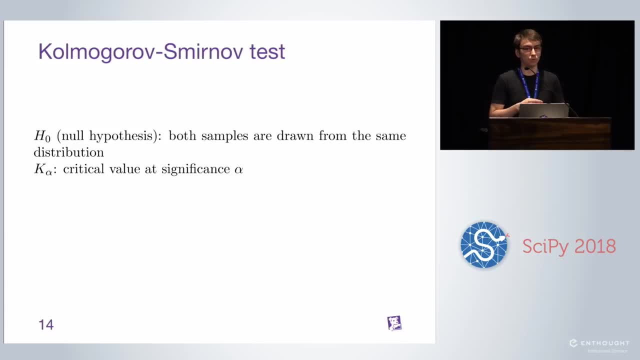 that is usually tabulated, or you can also compute it from the Kolmogorov distribution And then, if the value that we computed in the previous slide is lower than negative, you would have a critical value at significance alpha, And when you do that you would have a critical value. that's usually tabulated. 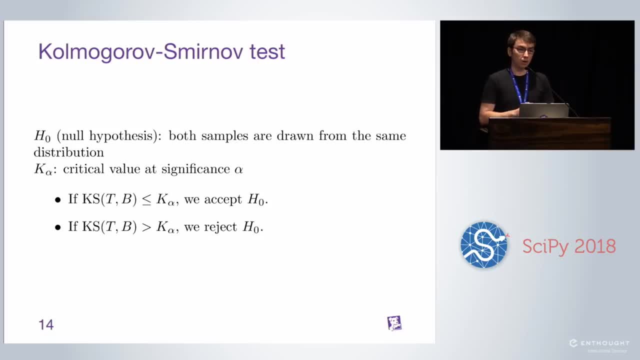 So if you can compute from the Kolmogorov distribution, you would have a critical value at significance alpha. this critical value we would accept H0. Otherwise we would reject the null hypothesis. So we can use this to say whether or not the test distribution should be flagged as anomalous. 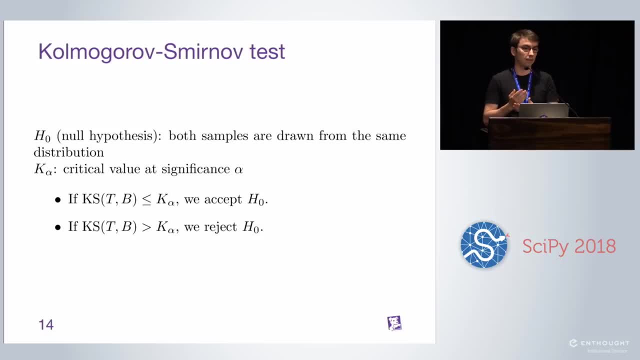 So if we reject the null hypothesis, we can say that the test distribution is anomalous. However, this only answers a yes or no question, and we might be interested in having a measure of how anomalous the distribution is. Maybe we have different distributions or we have timeframes. 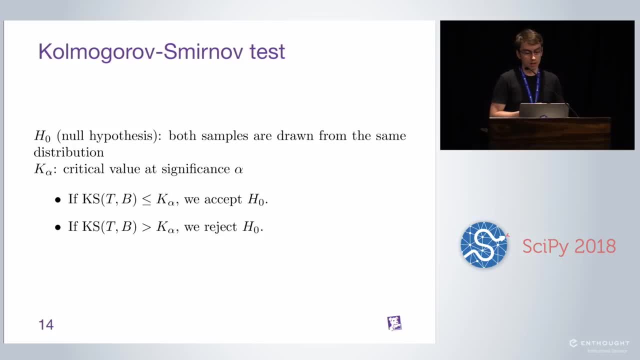 and we want to pinpoint the most anomalous timeframes or distributions. And we can actually easily do that here by simply keeping the case value, the number between 0 and 1, which is the absolute difference between the cumulative distribution functions. And the great thing, 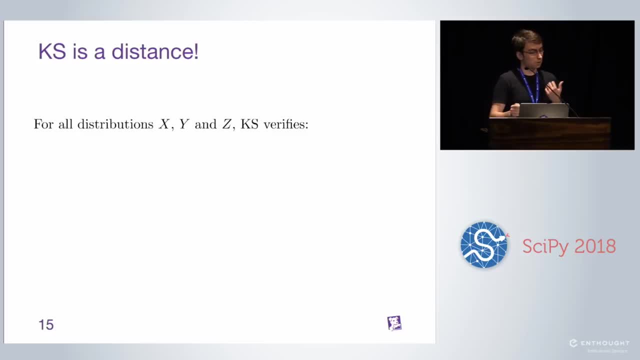 about this case value is that it is a distance. So if you have x, y and z, three distributions, case verifies the non-negativity. It's 0 if, and only if, x and y are the same, There is a symmetry and we also have the triangle. 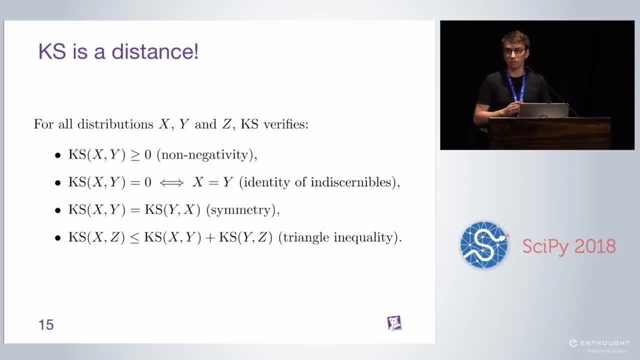 inequality. So the great thing of that is that now we have a metric space, So we have this abstraction where you can forget about the distributions and just consider that you have points in some metric space And you can apply all kinds of algorithms. So, for example, 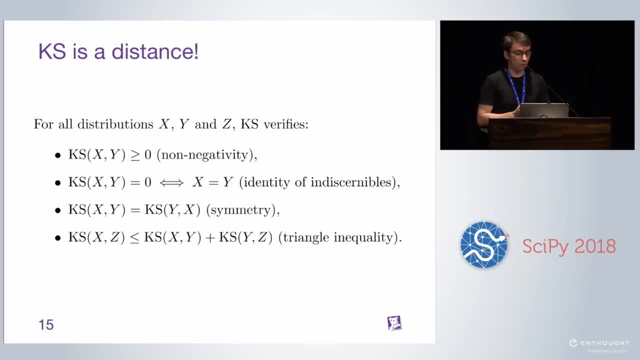 outlier, detection or clustering. What you could do, for example, is that if you notice that the point is far away from all the other ones, well, you can flag it as a non-negativity, But this one as anomalies. there is probably something wrong with that point, which is that 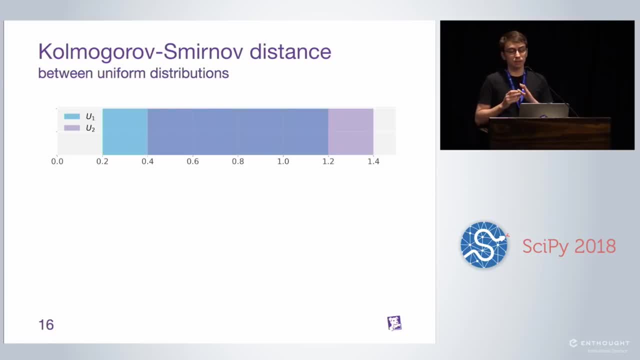 distribution. However, we still need to make sure that this commutative smear of distance is strong enough, rich enough, so that it will catch exhaustively all the anomalies that we're interested in. So we need to understand how this distance works. What we can do is looking at what 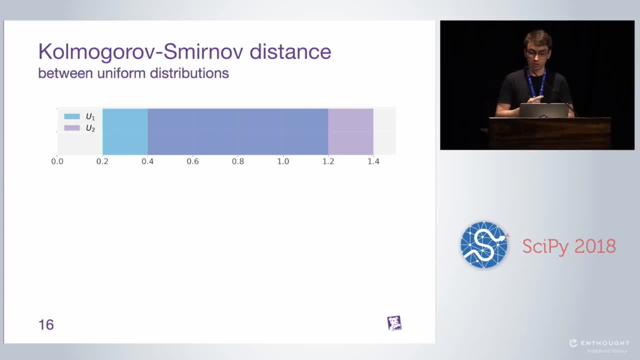 it looks like on some basic distributions. So here we have uniform distributions u1 and u2.. They are shifted from each other. If we plot the cumulative distribution functions, we get that And we get the common gross mean of distance. this way Now, if we shift one uniform distribution with regard to the other, 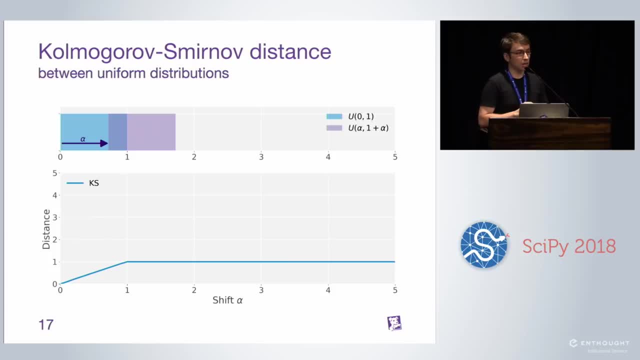 we can plot the distance as a function of the shift, And what we see here is that it increases linearly until 1, and that 1, it plateaus and stays at 1, which makes sense because that distance is always between 0 and 1.. But the thing here is that it's not great, because we can't say how different the 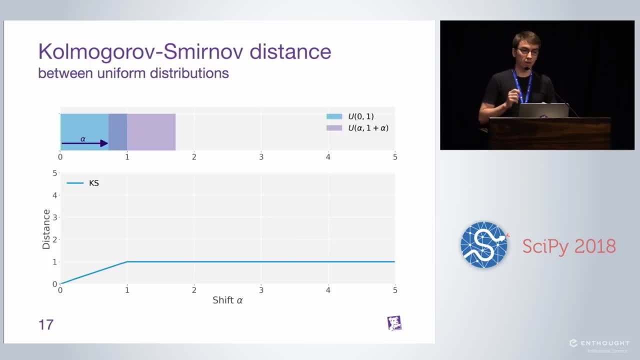 distance the distributions are When they are close, but beyond a given threshold, specifically when the uniform distributions are not overlapping anymore, we can't say anything anymore. We can say how far away they are from each other. So we need another distance. 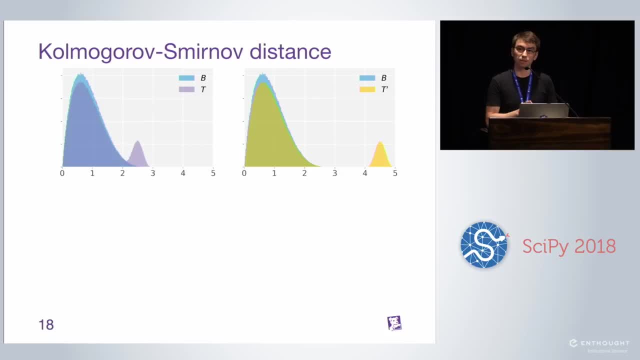 Yeah, so you might imagine that this uniform distribution case is an artificial case, But in practice we could have this. So we have three distributions here: b, which is again the baseline, and two test distributions, t and t prime. We see the small bump on the right. For t prime the bump is further away. We could imagine that in practice. so we have those web. 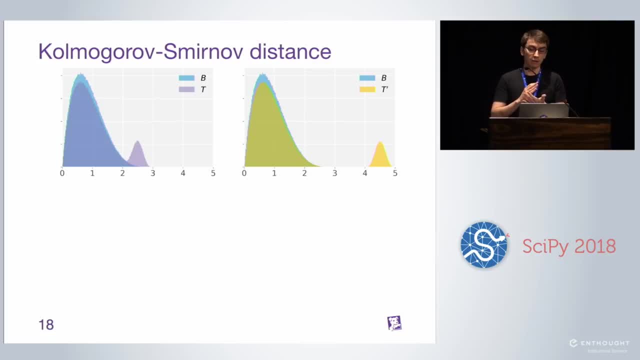 requests And for a small portion of the web requests we have a higher latency. This is the small bump, And what we'd like to see here is that t prime should be further away from b than t. However, if we look at the cumulative distribution functions and the case, 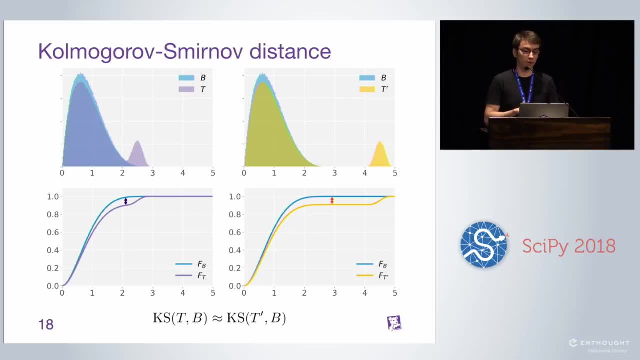 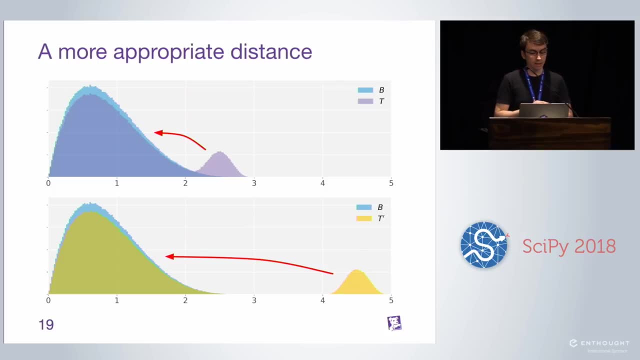 distance. this is not what we see. Basically, the distance is the same for in both cases. So what we need is a distance that's more appropriate for this kind of case of cases. So we need a distance that somehow uncovers the fact that there is more work involved to make t match b, to make t prime- sorry- match b, rather than to make t match b. 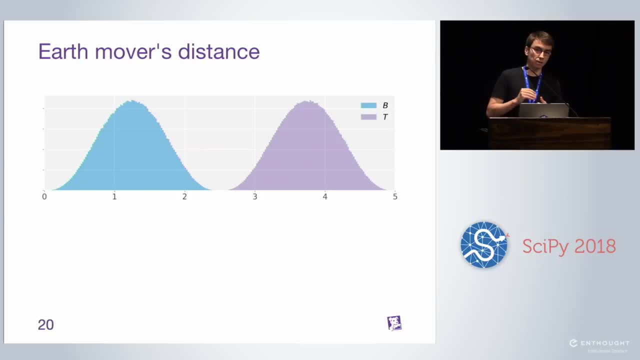 And this is actually the idea- between the Earth's movers distance. So we can imagine that our two distributions here are hips of Earth and that our job is to make one distribution match the other by moving this Earth from one place to the other. So when we do that, we define a mapping gamma, And this mapping gamma of x and y is the amount of Earth that we move from x to y And the. 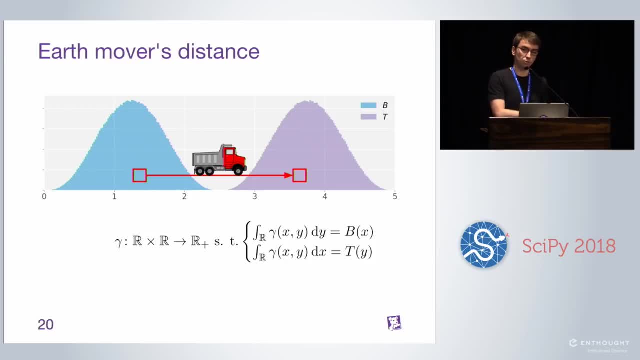 conditions on the right just translate the fact that we start with the b distribution and with the t distribution. We can consider all such possible mappings And for a given mapping we can look at the work that is involved in in moving the distribution following the mapping. So basically, this will be the distance, the amount of Earth that we're moving, times, the distance over which we are moving, and we sum over everything. 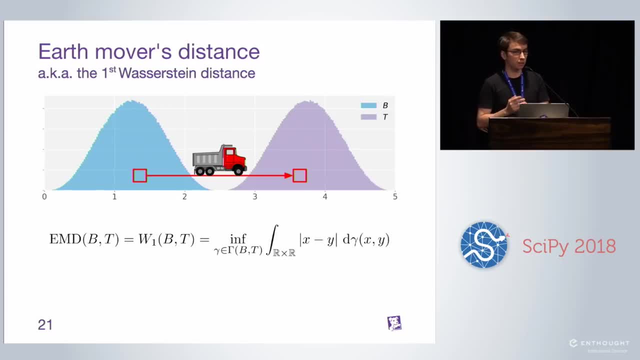 And if we consider the mapping that is the most efficient, that is to say that involves the least work, we define the Earth's movers distance. So, in other words, the Earth's movers distance is the minimum work that is involved when we move one distribution to the other where work is. 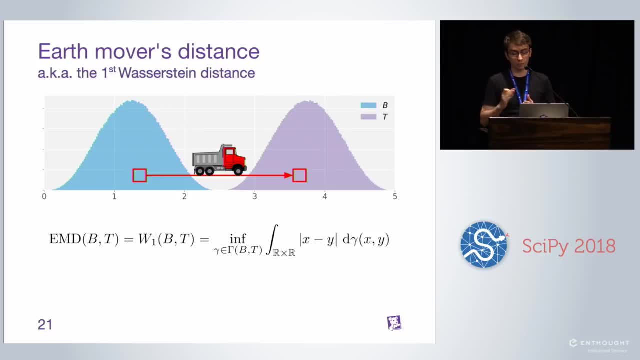 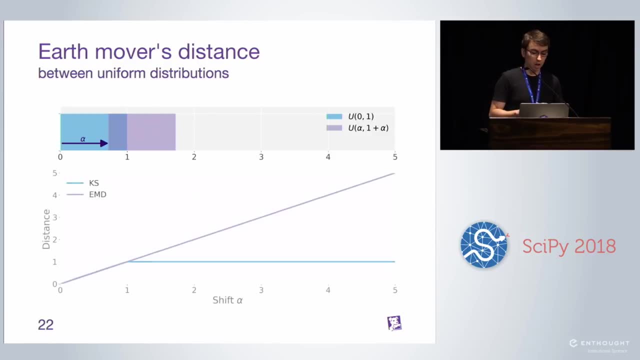 the amount of Earth that we move times the distance over which we move it. So now, if we look at the Earth's movers distance and our uniform distributions, we can see that the Earth's movers distance keeps increasing linearly, even when the support of the distributions are not overlapping anymore. So there is an issue, though, with this Earth's movers distance is that it is an infimum by definition and it's probably going to be quite expensive to compute. However, in the one-dimensional 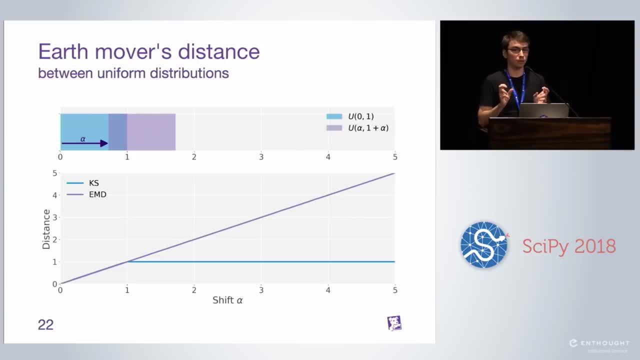 distance. we can see that the Earth's movers distance keeps increasing linearly, even when the support of the distributions are not overlapping anymore. So there is an issue, though, with this Earth's movers distance is that it is an infimum by definition, and it's probably going to be quite expensive to compute. However, in the one-dimensional 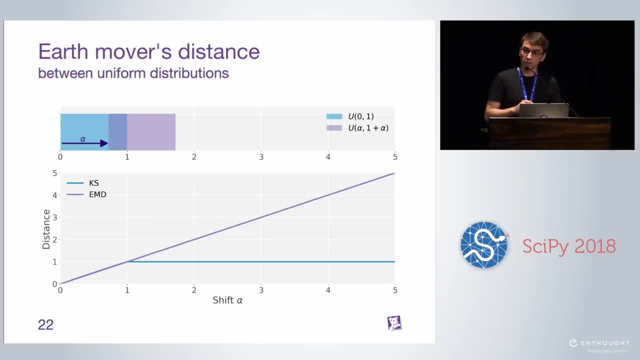 going to be quite expensive to compute. However, in the one-dimensional case, there is another way to define the Earth's movers distance, which is using the cumulative distribution function. So if we look at the cumulative distribution functions of both those distributions, we can: 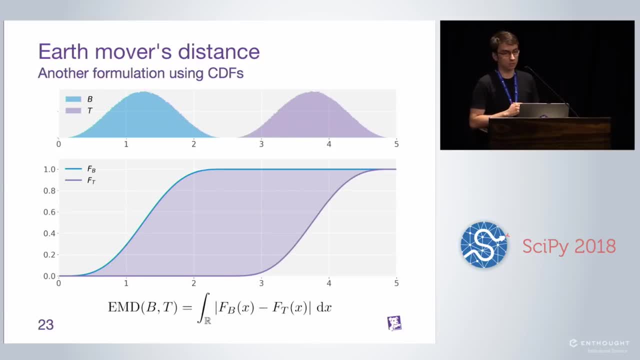 prove that the Earth's movers distance is equal to the area between the cumulative distribution functions, So this makes it much easier to compute. This is actually the way how we implemented it and what we contributed to SciPy, And so another great thing is that we 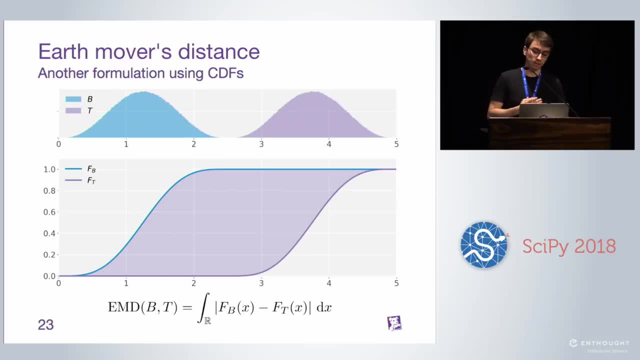 have an intuitive way of understanding what the Earth's movers distance is here. So on the bottom graph here, if you flip the x and y-axis, you will get the quantile functions of both distributions, But you're not going to change the area. 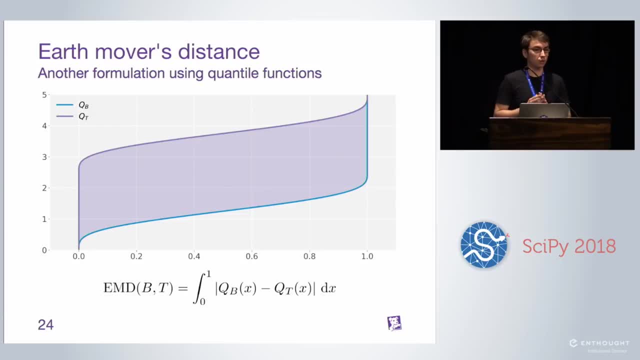 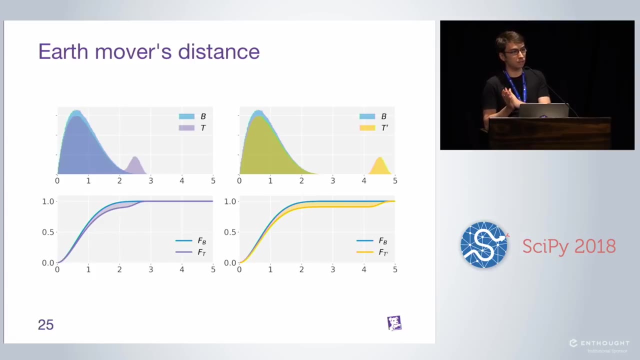 between the functions, which means that we can also compute the Earth's movers distance using the quantile functions. So now we can look at what the Earth's movers distance looks like on those examples. And now it's clear that, using the fact that it's the area between the cumulative distribution, 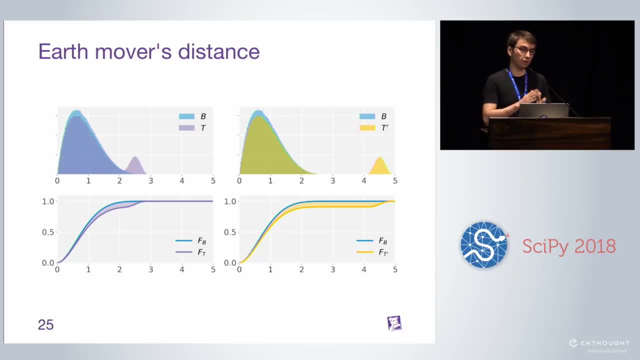 functions, we're going to have a higher distance on the right than on the left, So this distance seems better than the Kolmogorov smear of distance to catch these kind of anomalies. However, there are still some cases for which we still don't catch the deformation or the anomaly. 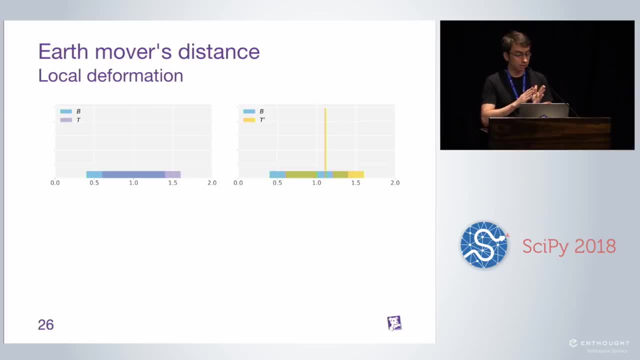 So here on the right we have two uniform distributions And on the left, sorry, we have two uniform distributions, And on the right we generate t prime by accumulating mass in a single point. Now if we plot the cumulative distribution functions of those, 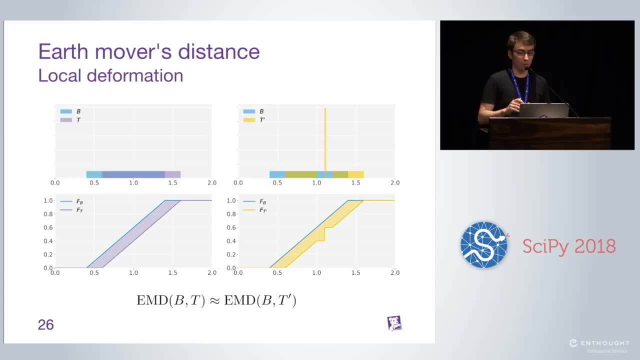 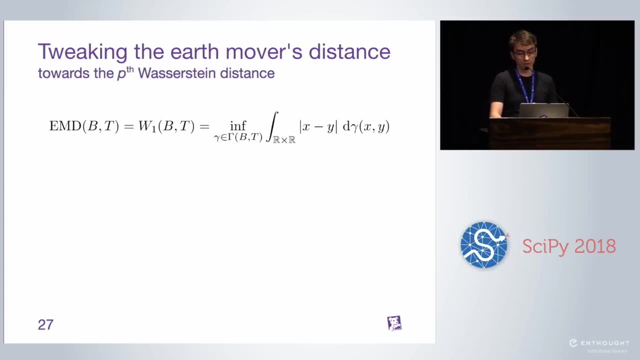 and we look at the area, it's clear that by doing a bit of geometry we have almost the same value here. So we are not catching the anomaly in this case, But we can work from the Earth's movers distance, which, once again, is also the first fast-threshold distance. 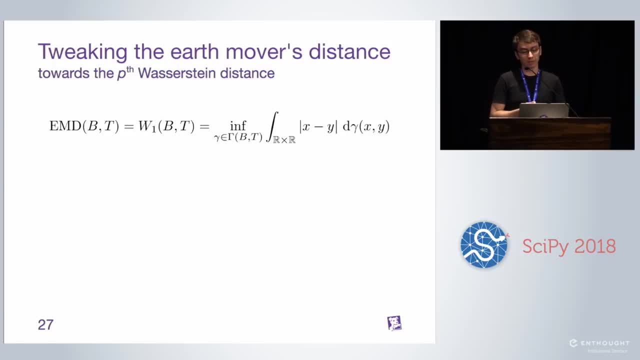 So as a reminder, so this is the formula for the Earth's movers distance, Which is also the area between the quantile functions. What we could do here is, instead of taking the absolute difference between x and y, we could take that absolute difference to the power p. 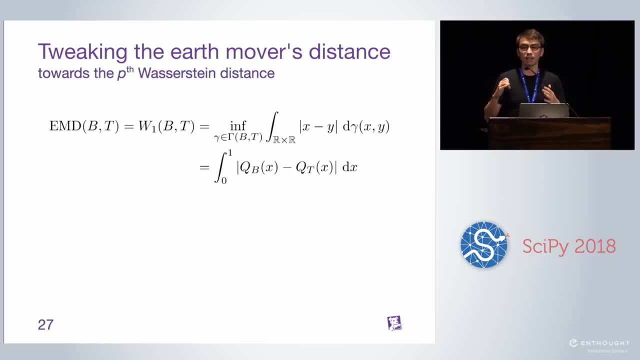 So we give actually more weight to the, we penalize more the larger differences And if we do so, we define a new family of distances which is actually the family of Vassarstein distances, And the piece of Vassarstein distance is defined as this: 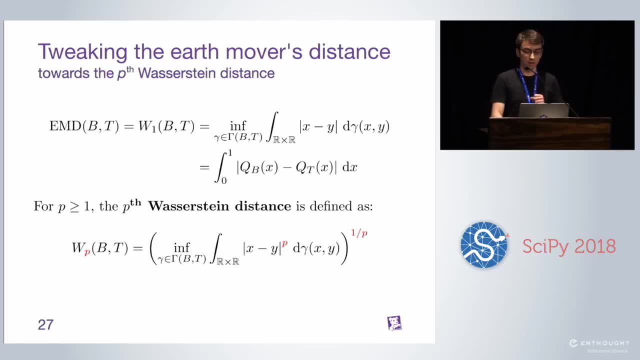 And the great thing is that we can still prove that we can compute this distance from the quantile functions. So it's still easy to compute in the one-dimensional case. So if we look at this last line, we modified the formula with the quantile functions. 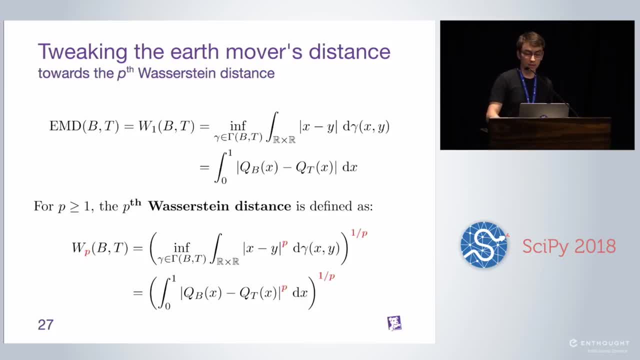 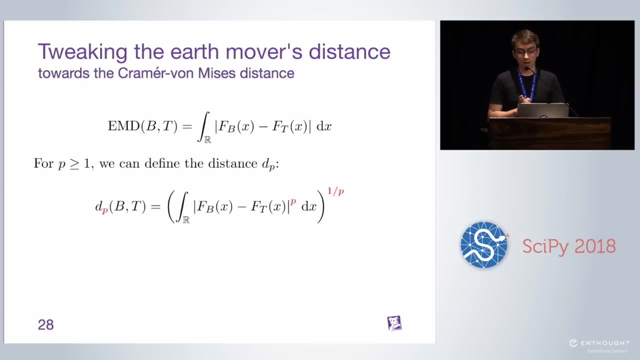 What if we do the same thing with the cumulative distribution functions? So what if we start with this and we decide to build this new family of distances? Well, we define- actually those are also distances- statistical distances, And if we take p equal to 2, we define the Cramer-von Mises. 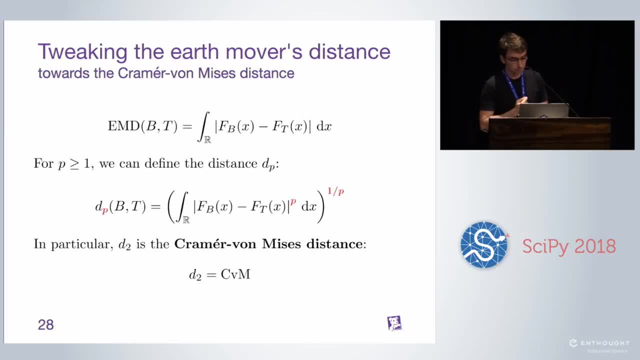 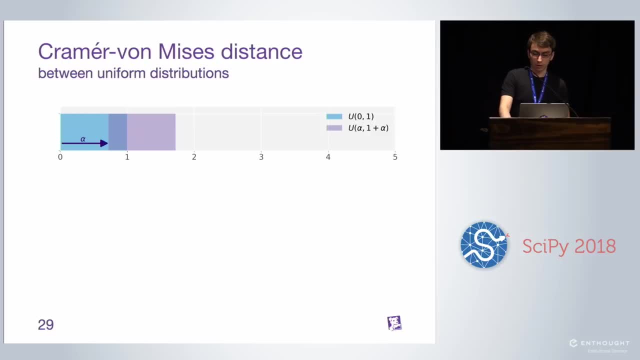 distance, which is sometimes just called the Cramer distance. It's actually related to the Cramer-von Mises statistical test. So if we look at the Cramer distance with our uniform distributions, this is what we would get. So basically, it increases like a square root. 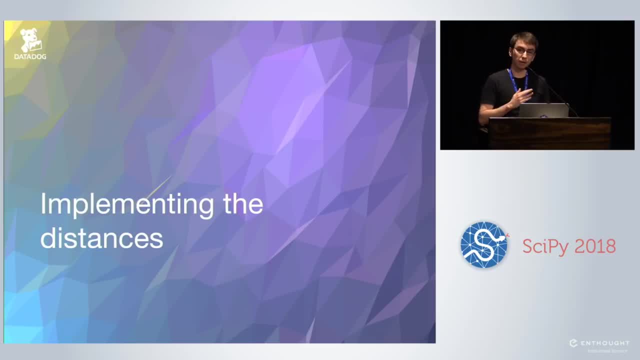 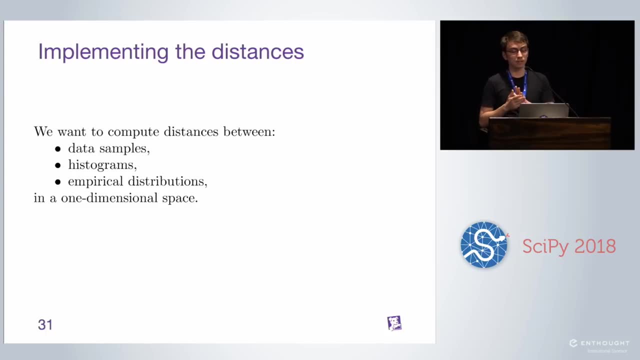 So, now that we have the intuition and the theoretical background behind all those distances, we need to implement them And, in our case, we want to compute distances between practical data, not between theoretical distributions. So we need to compute distances between data samples. 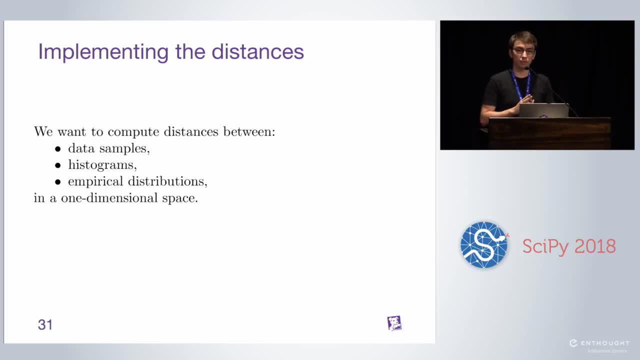 histograms, empirical distributions, and all of this in one-dimensional space, And what we can do is encode all of this data with values and weights. So if you work with data samples, the values are basically the values of the data samples. 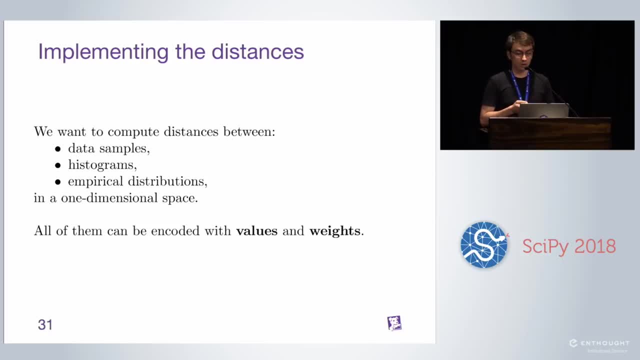 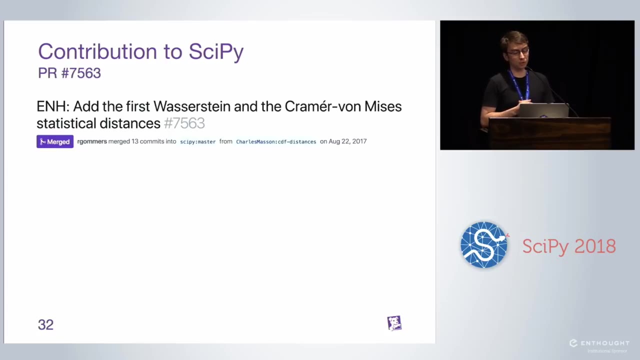 And the weights might be the number of occurrences. For histograms, you could have bin positions, which are the values, and the height of the bins, which is the weight, And we can do the same thing with the empirical distribution. So we implemented those distances. more specifically, 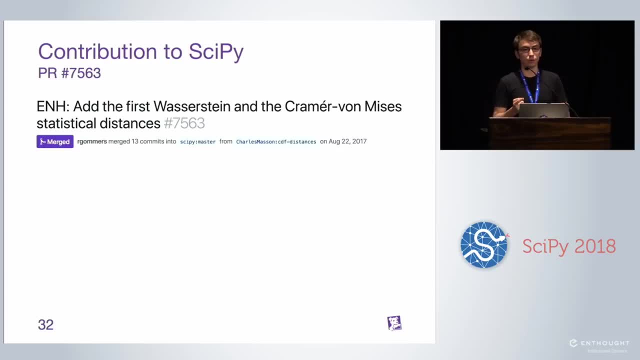 the Vasterstein distance and the Cramer-von Mises distance. The Kolmogorov-Milnov distance is already implemented in SciPy, So up here it got merged Last summer And now you can basically use those distances in SciPy. 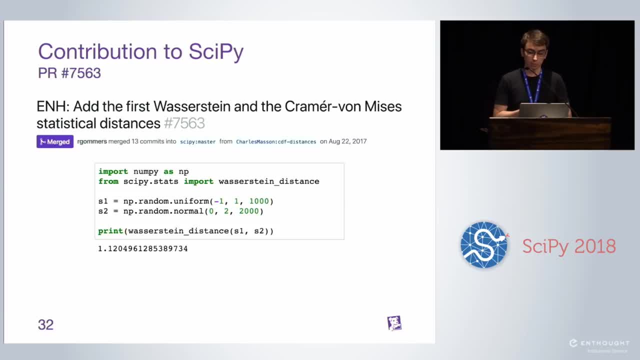 So here we generate two samples from uniform and normal distributions. We can compute the distance between those samples And if you work with weights, so maybe we have a histogram with the height of the bins. that are the weights. here you can also compute the distance between those histograms. 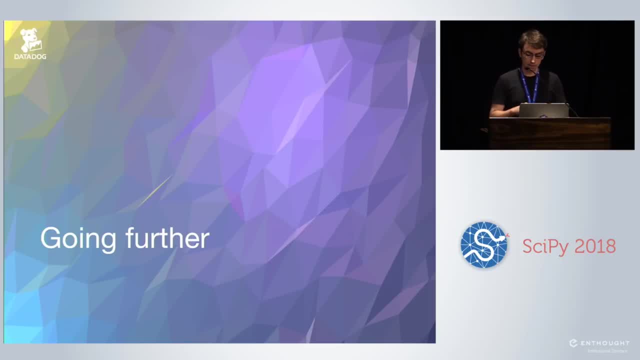 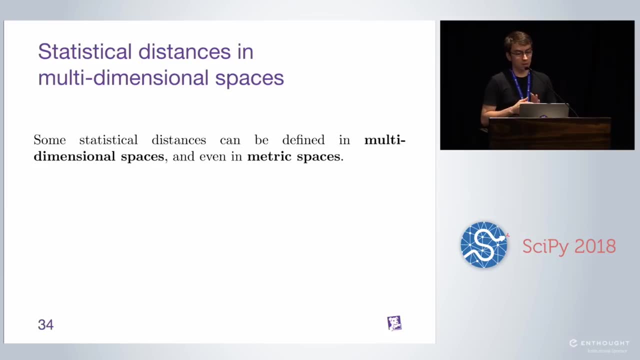 So we can do actually much more with statistics. So the first thing is that- statistical distances. I focused on specific cases, especially on the one-dimensional case, But there is actually much more that we can do. So the first thing is that: statistical distances. 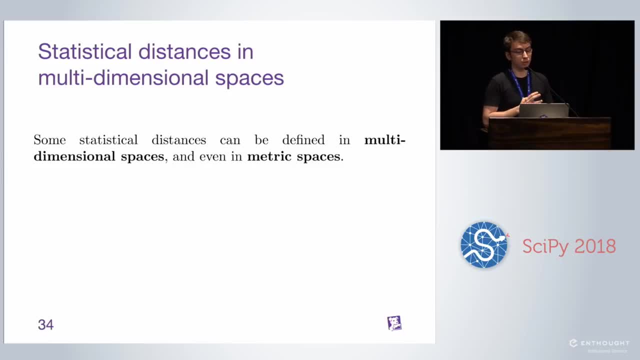 can be defined for some of them in multi-dimensional spaces and also in metric spaces, And applications of that are pattern recognition, image processing. So, for example, if you work in a two-dimensional case, two-dimensional space, You can actually use the Earth's movers distance. 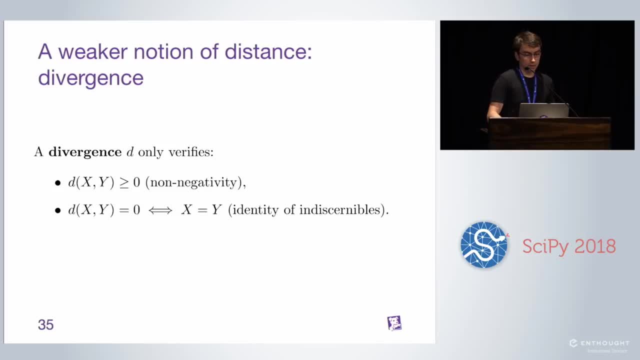 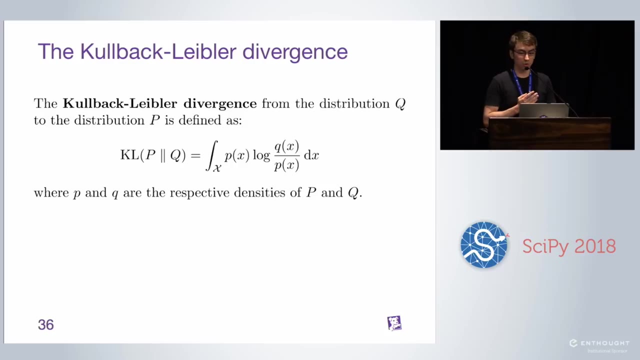 to say how close two images are. There is also a weaker notion of distance, which is the divergence. The divergence only verifies the non-negativity and the fact that it is 0 if, and only if, x is equal to y. And one specific divergence is the Coulbert-Claibé divergence. 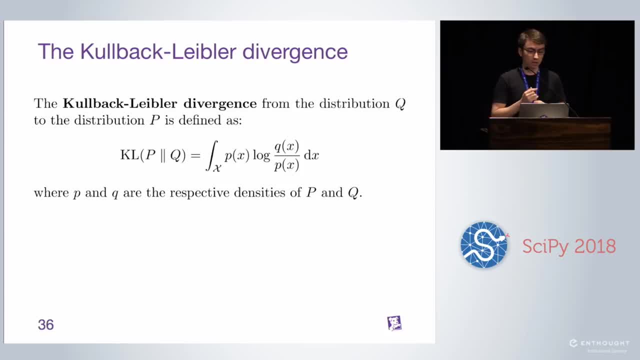 between two distributions, which is defined as this, where small p and small q are the respective densities of P and Q, And we can show that solving the maximum likelihood estimation problem is equivalent to minimizing the cool-back liability divergence. So the maximum likelihood estimation 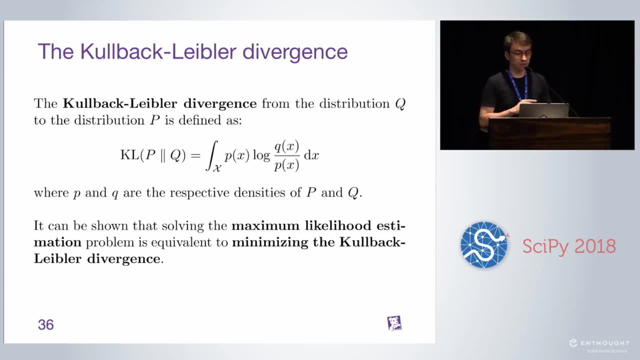 is used in a variety of programs and machine learning models, And when we do that, we are actually just doing the same thing as minimizing the cool-back liability divergence, which is this value. So if we look at the formulation of that divergence, we can see that we look at the densities at specific points. 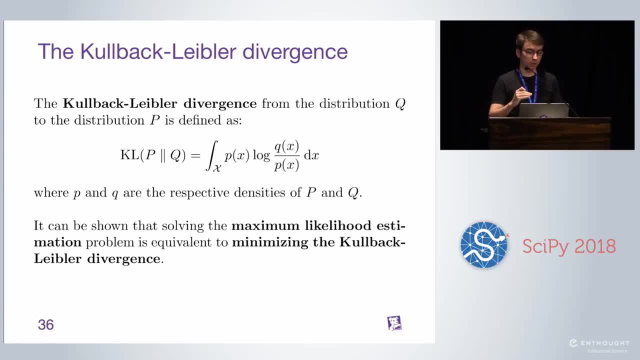 So we look at how different we have this ratio between Q and small q and small p, And then we sum over everything, which means that if we have distributions that have high densities in very small, very close areas, but not exactly in the same area, 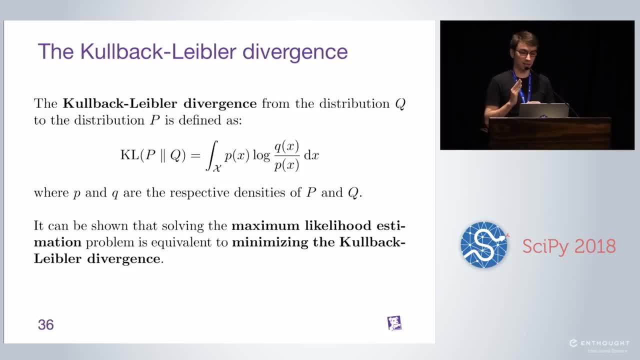 the cool-back liability divergence won't be able to catch that, because it only looks at the ratios between the densities in a single point and then sum over everything, And this is actually something, an issue that we saw in the literature for some machine learning. 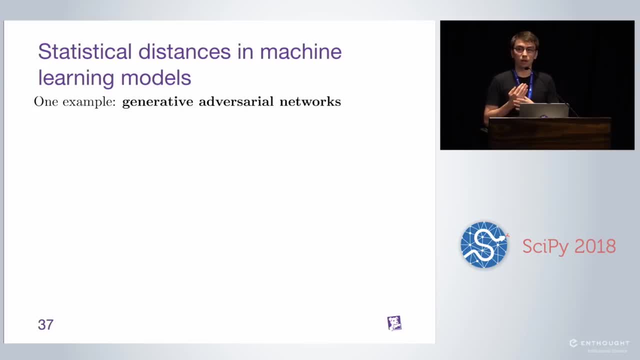 model, especially generative adversarial networks. So I won't go too much into details, but basically generative adversarial networks are machine learning models. They are machine learning models that generate data and that can be used to generate data that would look real. 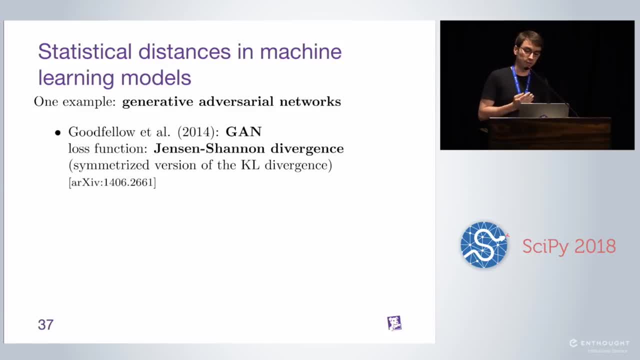 So the first publication that we saw about generative adversarial networks was in 2014.. And at the time, the last function that was used is the Jensen-Shannon divergence, which is a symmetrized version of the cool-back liability divergence. 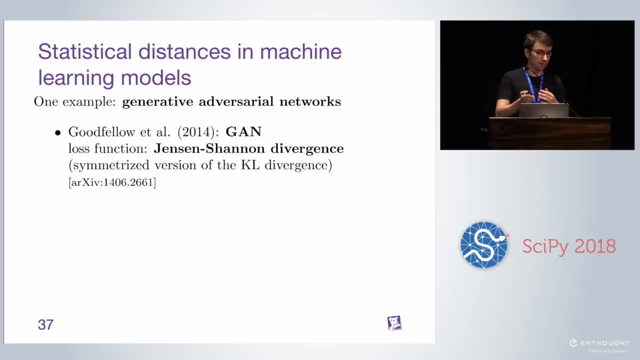 And so one issue that we saw is that, as I explained in the previous slide, sometimes we have images that are very close. Well, actually, we have distributions of images when we generate images with these models that are very close but not exactly the same. 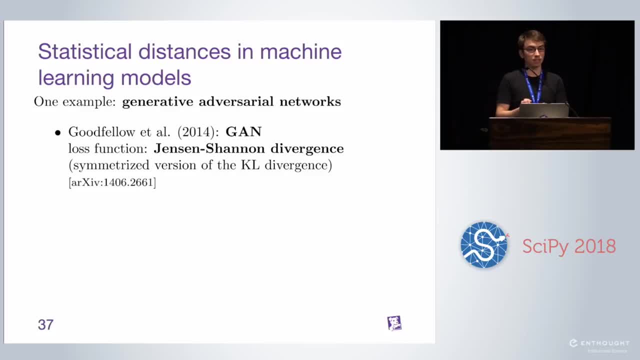 And this loss function is not able to catch this, to model how close those distributions are. And that's why a few years later we saw the Wasserstein generative adversarial networks where the loss function is not the Wasserstein distance, And this was partly to the benefit of the machine learning. 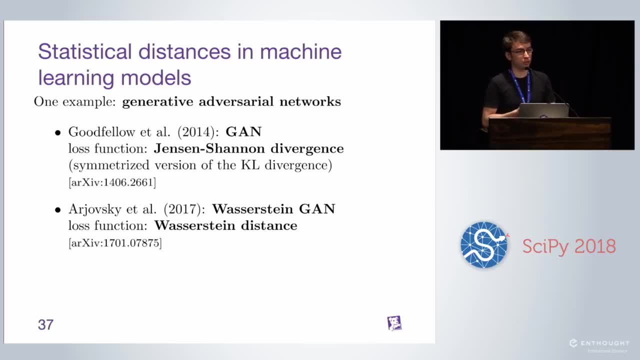 model. It was to solve the issues that we saw in the previous models and the previous loss functions, And a few months later we saw the Cramer generative adversarial networks. Now, in this case, we use the Cramer distance. 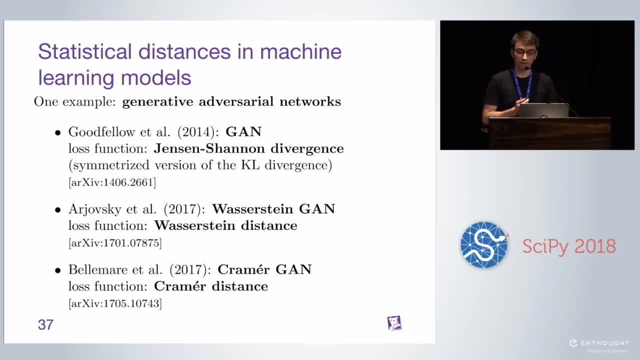 which also solves some other issues that we have with the Wasserstein distance, including some bias that we might have when we work with samples, And so this is also a reason why statistical distances got quite common. It's only used in the literature over the past years. 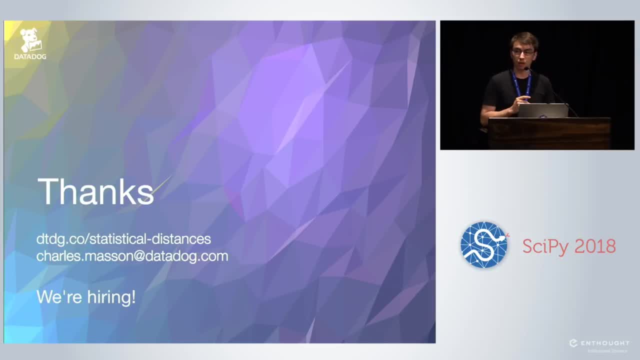 So that ends my talk. So we have a blog post with more details about the statistical distances, with references and also with animations so that you can try for yourself and compute distances between some distributions. If you have any questions or feedback, you can get in touch with me. 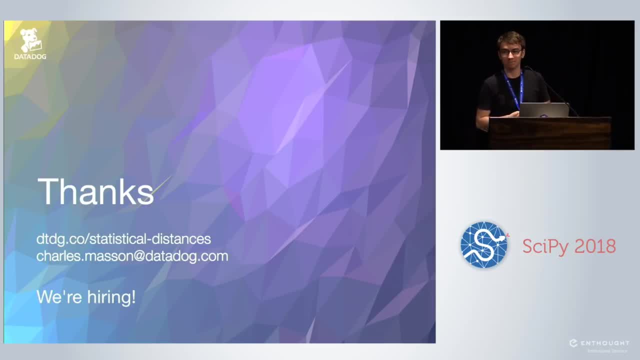 And, by the way, if you're interested, we're hiring. Thank you, Thanks, Charles, That was great. We have time for a few questions. Again, please ask only one question and phrase it as a question. I'll take the mic to this side of the room. 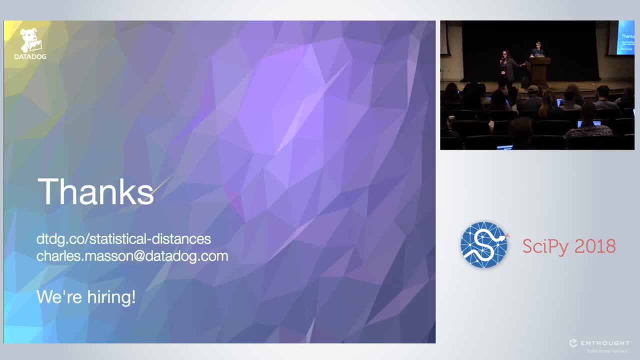 And for this side of the room again, please line up and I can signal to you from the line Questions. Thank you, Charles. Very interesting talk. When you do the sample computation of Lester-Stein distance, for instance, you do this quantile differences. 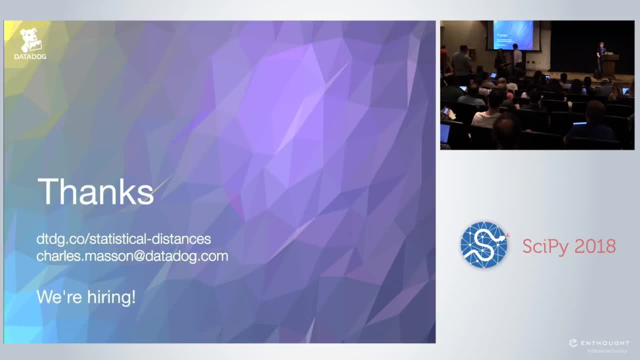 Interpolation between quantiles for integration. does it influence the value of the distance And, if so, what type of interpolation have you chosen? So we don't actually need to do an interpolation to compute the distances. So what we would do is work in with the empirical distributions. 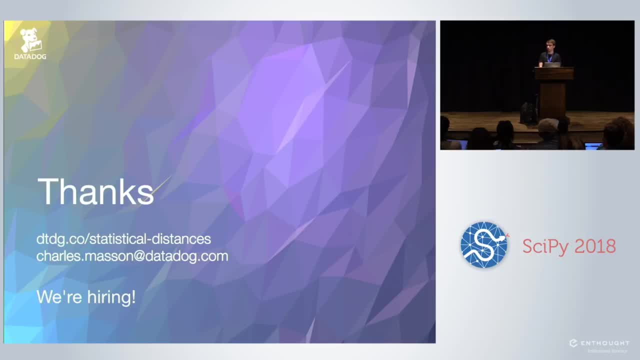 And we can actually compute the distances from the empirical distributions. So we would have steps basically in the distributions but we don't need to do any interpolation between the points that we have. So we don't need to, but we can. 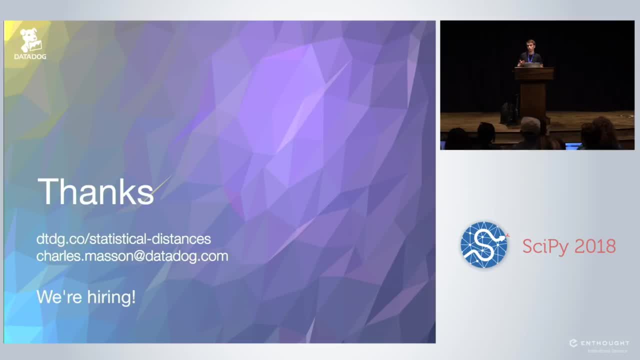 We could, yeah, But when we work with empirical data, we don't need to. I don't think we need to. Other questions? Oh, Maybe, just as an easy example, you brought up with the very static system behaviors in the plot. 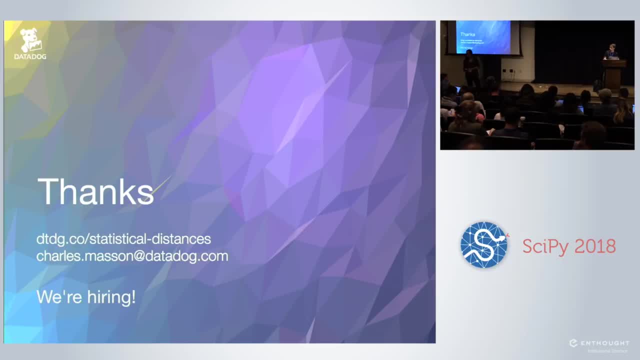 Have you guys also applied a bit more non-static system behaviors and checking the anomaly based on your statistical distance? So, yeah, I think that's a good question. Yeah, So on real data rather than Yeah, Some real data actually just varying over the time. 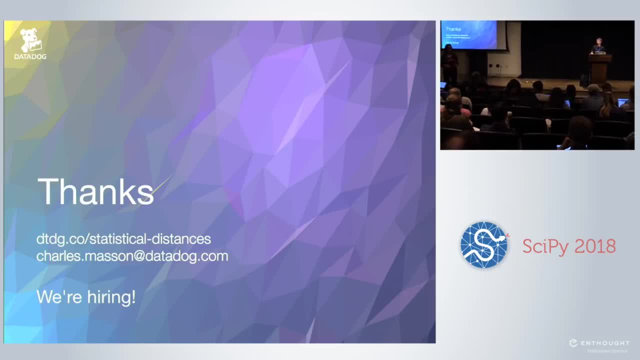 and system degraded and there is some changes in the system. So they are not necessarily anomalies, but yeah. So I think it all depends on how you actually use the statistical distances. I'd say this is more about the low level of your algorithm. 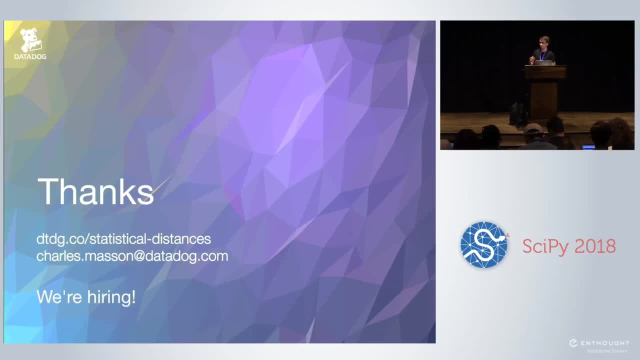 And then it all depends. It all depends on how you would actually use that. So if, for example, you want to be resilient to shifts over time, you would probably want to take a baseline that is far in the past to make sure that you're not adjusting to the latest behavior. 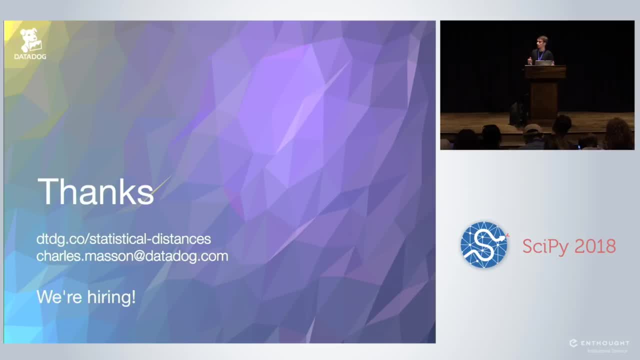 And this is something that we actually do. But, yeah, for the statistical distances by themselves, I think, yeah, there are more just breaks that you can use the way you want in your models. OK, Thank you, Thank you, Thank you.